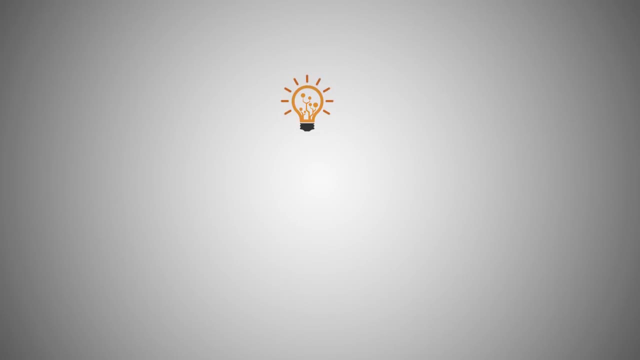 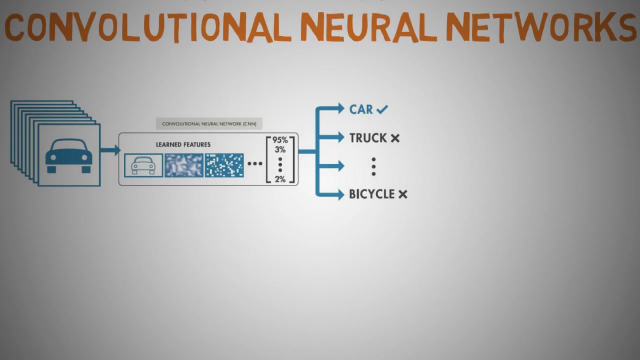 Hey guys, and welcome to another fun and easy machine learning tutorial on Convolutional Neural Networks. So what are Convolutional Neural Networks and why are they important? Well, Convolutional Neural Networks or ConvNets, also known as CNNs, are a category of neural 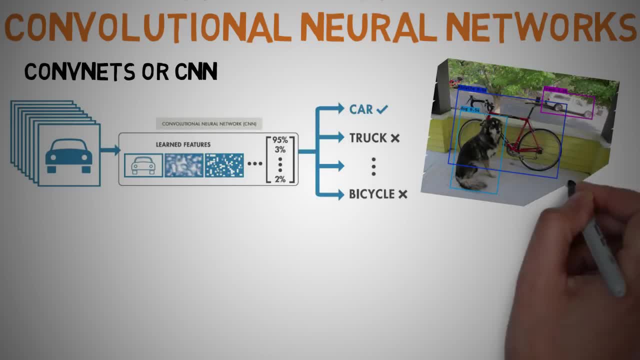 networks that have proven very effective in areas such as image recognition and classification. ConvNets are very successful in identifying faces, objects and traffic signs. apart from powering vision in robots and self-driving cars, A ConvNet is able to recognize scenes and the system is able to suggest relevant captions, for example, a girl playing tennis. 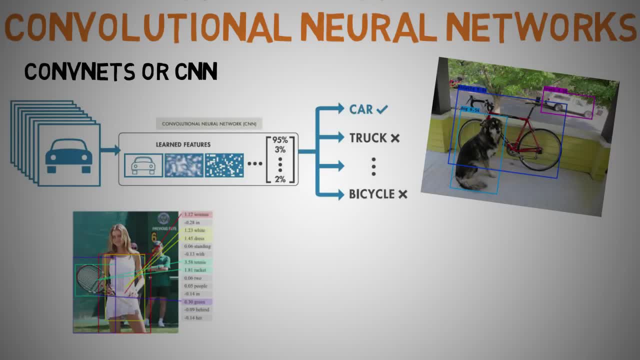 while this image shows an example of a CNN being used for recognizing everyday objects such as humans, objects and animals, There are also ConvNets involved in playing games such as Starcraft, Doom and Mario. CNNs are therefore an important tool for most deep 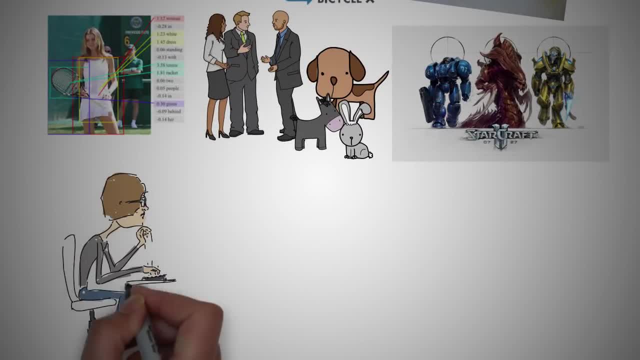 learning practitioners today. However, understanding ConvNets and learning how to use them for the very first time can be sometimes a bit daunting. But don't worry, you're in good hands here at Arduino Startups. If you are new to neural networks in general, I would recommend you check out my lecture on Artificial Neural. 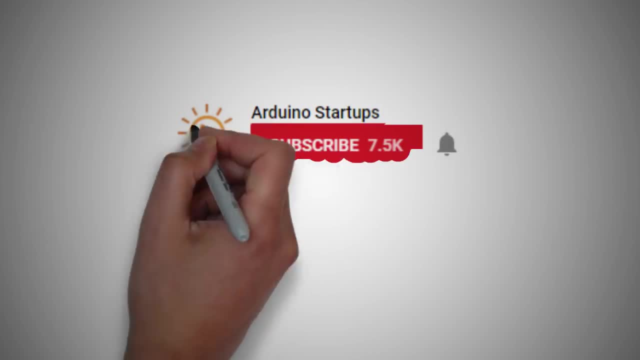 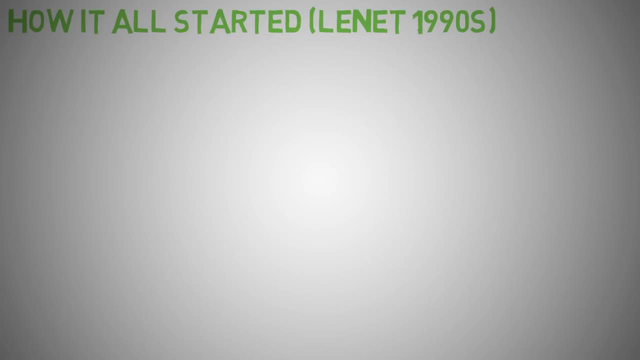 Networks and then return to this one. Please subscribe and click that bell icon to join our notification squad. Let's take a look at how it all got started. So LeNet was one of the very first Convolutional Neural Networks, which helped propel the field of deep learning. 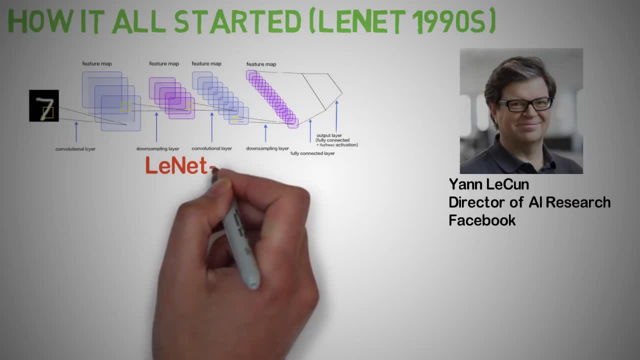 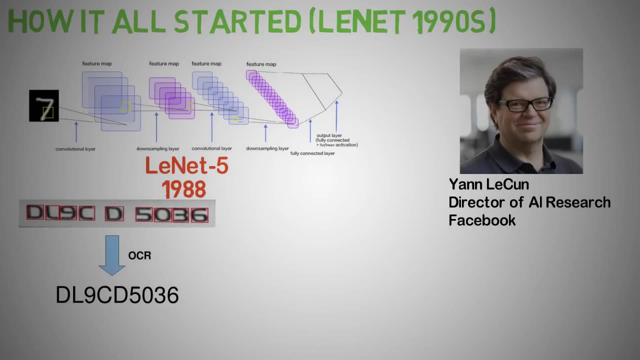 ConvNet Yann LeCun was named LeNet 5 after many previous successful iterations since the year 1988.. At that time, the LeNet architecture was mainly used for character recognition tasks, such as reading zip codes, digits and much, much more. Since then there was a pause. 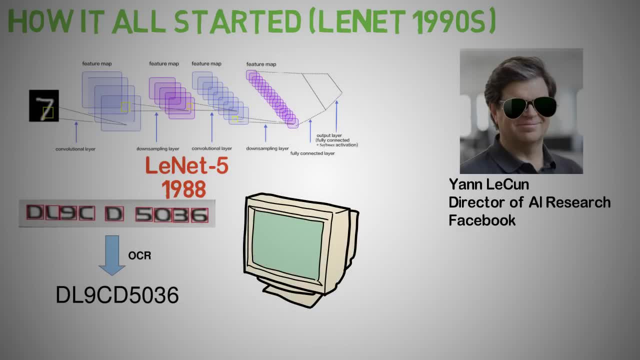 in the development of ConvNets and neural networks in general, and this is because of a lack of significant computing power at the time. ConvNets started picking up around 2012 with LXNet, amongst others. We'll discuss the various ConvNet architectures. 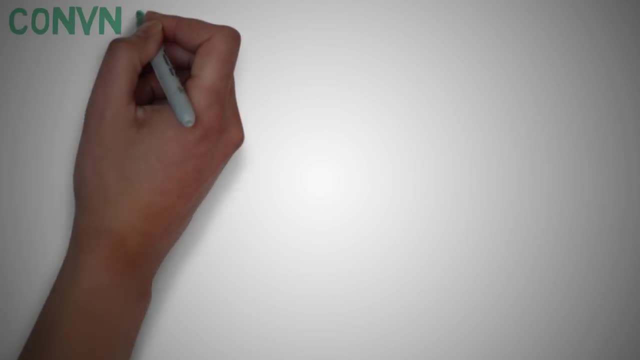 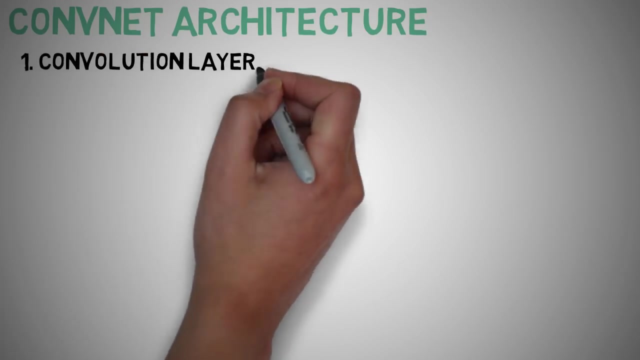 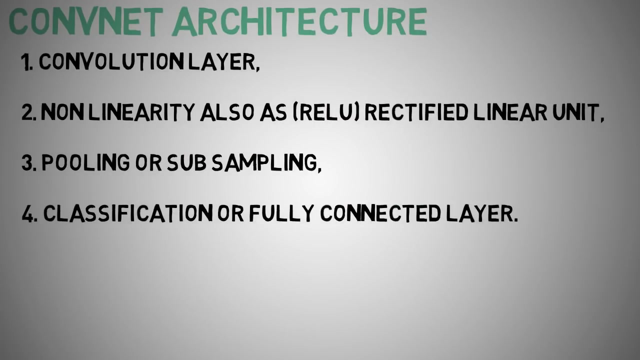 The ConvNet architecture. Let's take a look at the 4 main operations in the ConvNet, which are: The Convolution Layer, Non-Linearity, also known as ReLU, which is Rectified Linear Unit. Pulling or Subsampling, Classification, or Fully Connected Layer. These operations are the basic blocks of every CNN, so understanding how these work is a 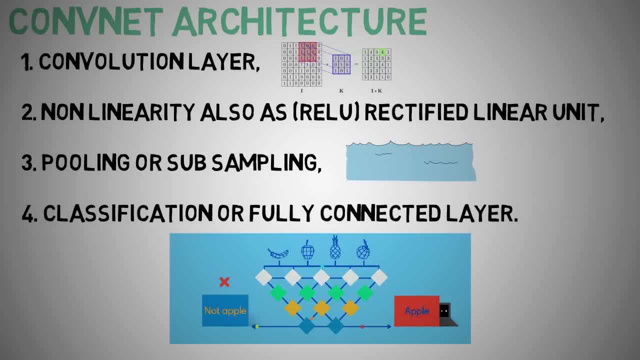 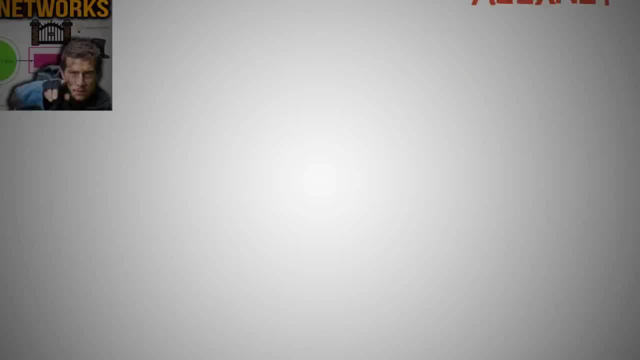 very important step in developing a ConvNet architecture. We'll first try to understand the intuition behind each of these operations as we progress through the lecture. Before we start with the main operations of CNN for image classification, let's recap some image processing 101.. Essentially, every image can be represented as a matrix of pixel. 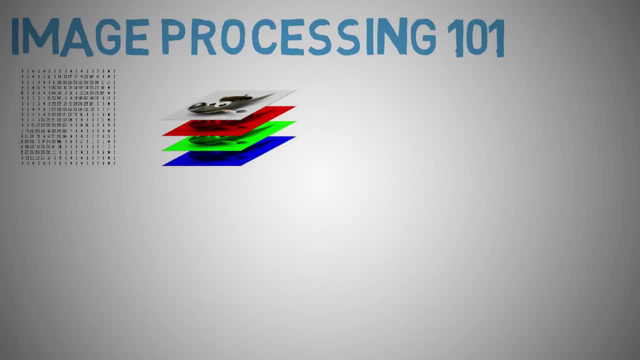 values. A channel is a conventional term used to refer to a component of an image. An image from a standard digital camera will have three channels: red, green and blue. This means that the image will be represented as a matrix of pixel values. A channel is a conventional term used to refer 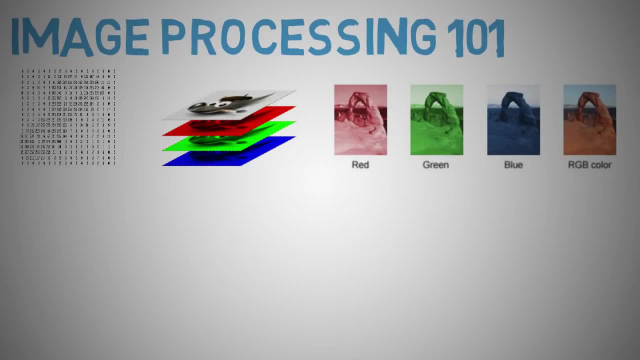 to a component of an image. An image from a standard digital camera will have three channels: red, green and blue. These zwrt channels represent the image. You can imagine those channels as 3, 2 dimensional matrices stacked over each other, One for each. 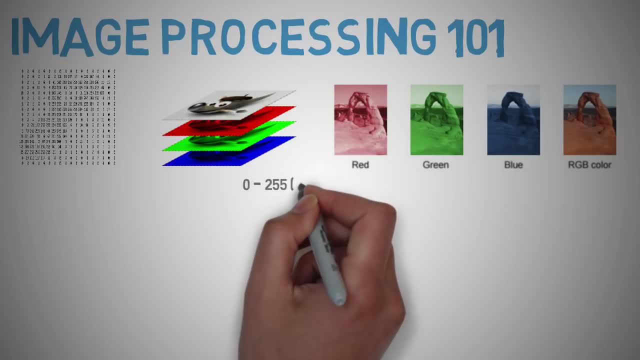 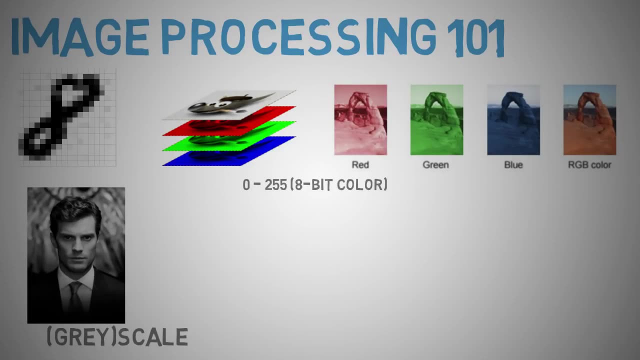 colour, Each having pixels in the range of 0 to 255.. A Grayscale image, on the other hand, has just one channel. For the purposes of this video, We'll only consider the grayscale images, so we'll have one single 2 dimensional matrix. 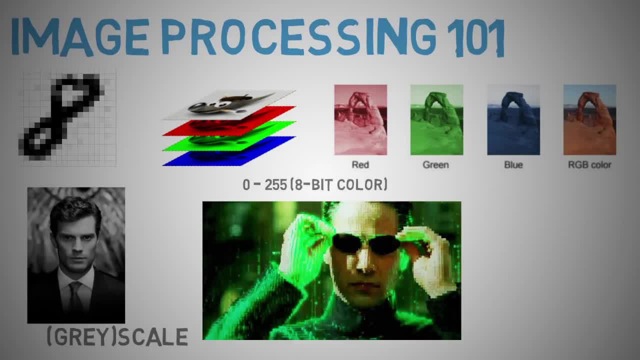 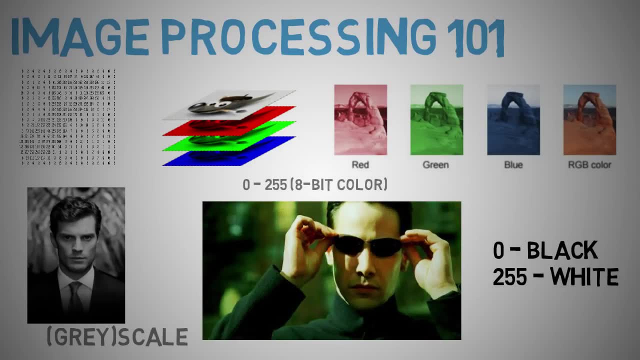 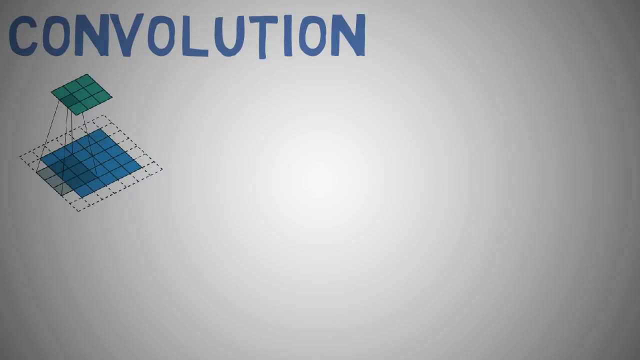 representing an image. The values of each pixel in the matrix will have a range from 0 to 255, as mentioned below before, where 0 indicating black and 255 indicating white. The convolution step ConvNets derive the name from the convolution operation. 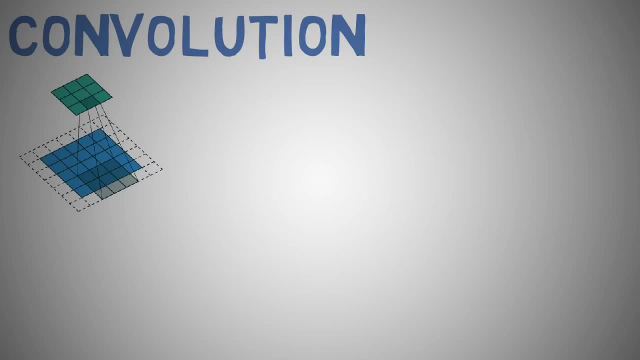 The primary purpose of convolution in the case of convnet is to extract significant features from the input image. The convolution operation preserves the spatial relationship between pixels by learning image features using small squares of input data. We will not go into the mathematical explanation of convolution here, but we will try to understand. 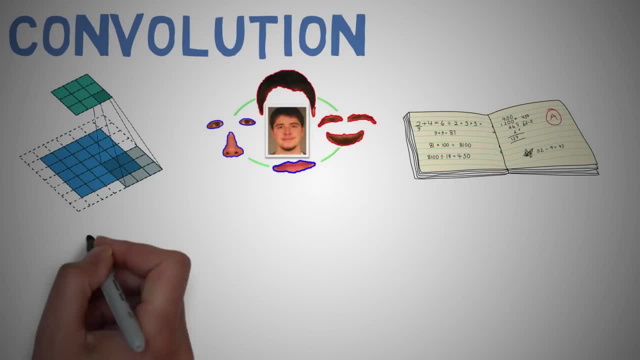 intuitively how it works over images. If you recall earlier, every image can be considered as a matrix of pixel values. So consider a 5x5 image whose pixel values are only 0 and 1.. We'll keep it easy and stick to binary images instead of a grayscale image. 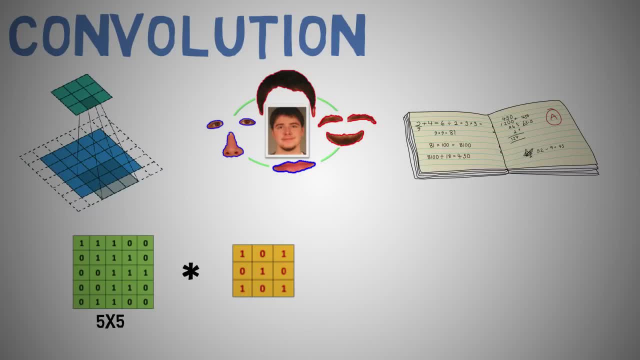 Also consider an arbitrary 3x3 matrix, also shown over here. Then the convolution of a 5x5 image and a 3x3 matrix can be computed as shown in this animation. Let's take a moment to understand how the computation is being done. 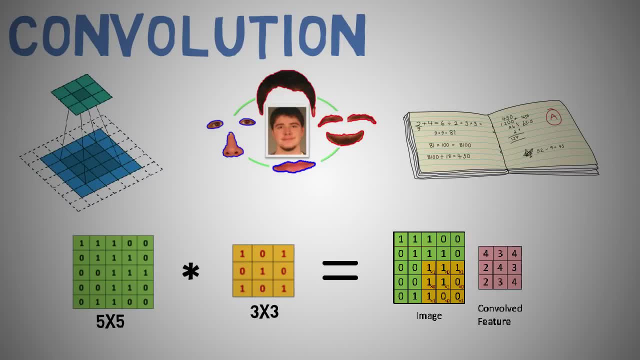 We'll slide the orange matrix over the original image green by 1 pixel, which is also known as a stride, and for every position we'll calculate the element-wise multiplication between the two matrices, And then we add the multiplication outputs to get the final integer, which forms a single. 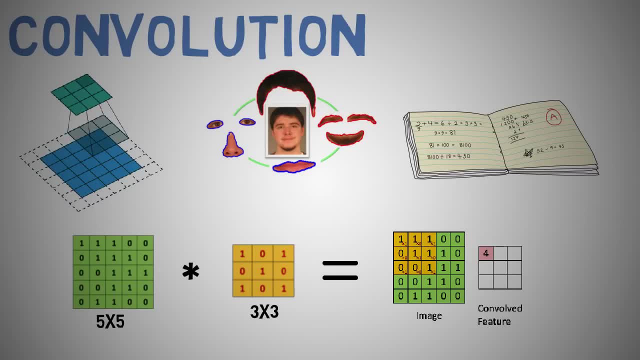 output from the output matrix in pink. Note that the 3x3 matrix sees only the part of the input image in each stride. So here we have 1x1, which equals 1.. And here we have 1x1, which equals 1.. 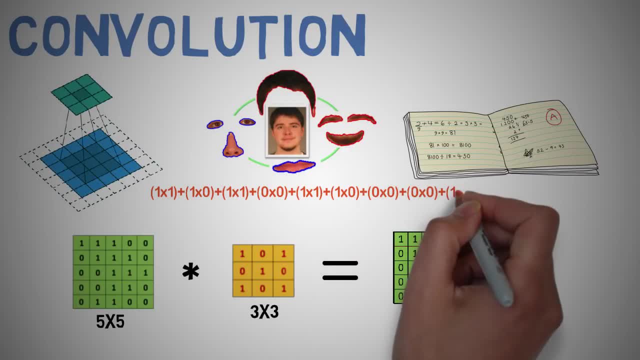 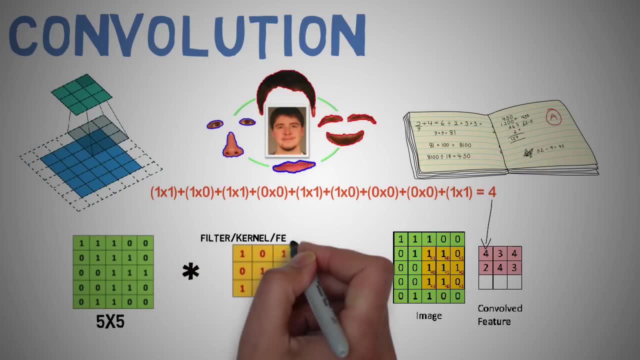 Plus 1x0, which equals 0. And then we continue adding all the products until you see that we end up with 4.. In CNN terminology, the 3x3 matrix is called a filter, also known as a kernel and also. 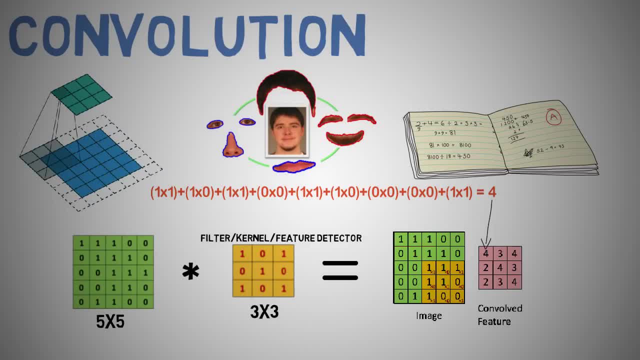 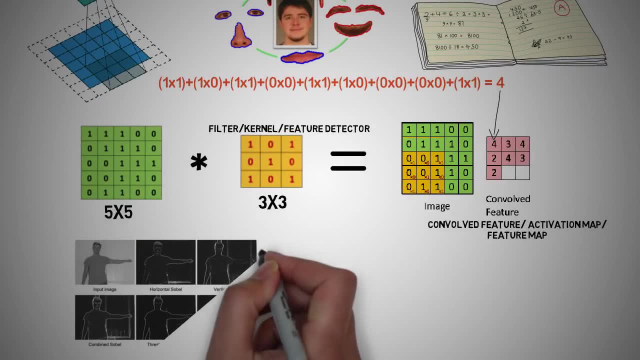 a feature detector. The matrix formed by sliding the filter over the image and computing the dot product is also called a convolves feature activation map or the feature map. It is important to note that filters act as feature detectors from the original input image. 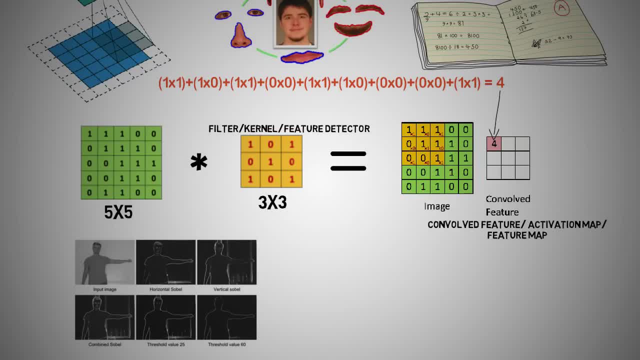 We can see over here that the function of the filter is the same as the function of the input image. So the different values of the filter matrix will produce different feature maps for the same input image. We can perform operations such as edge detection, sharpening and blur just by changing the numeric. 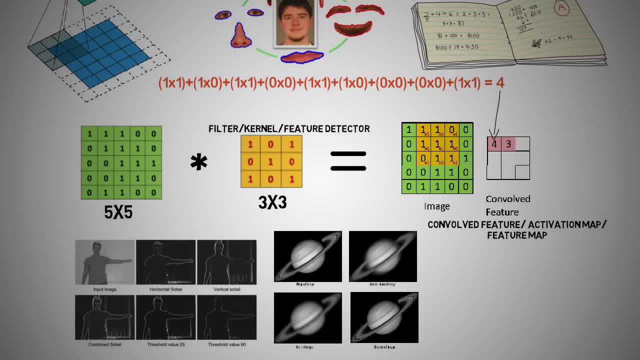 values of our filter matrix before the convolution operation. This means that different filters can detect different features from an image, for example edges, curves and much more. In practice, a CNN learns the value of these filters on its own during the training process. 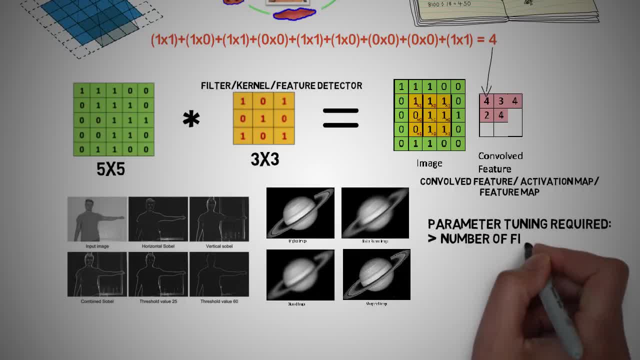 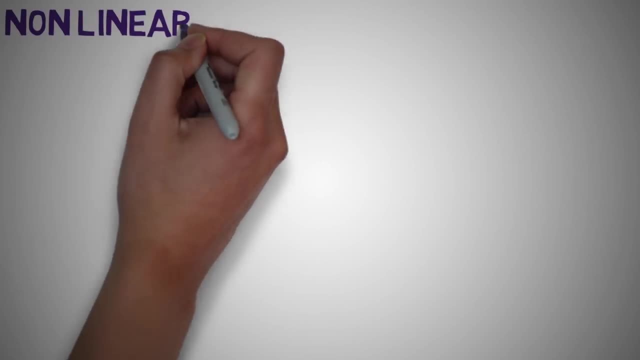 although we need to specify parameters such as the number of filters, the number of filters and the number of filters. The greater the number of filters we have, the more image features get extracted and the better our network becomes at recognizing patterns in unseen images. 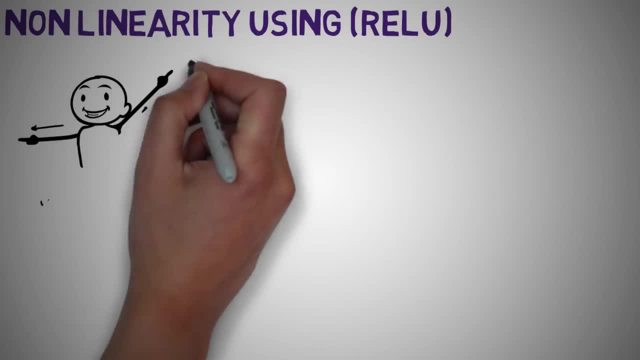 Non-linearity using ReLU. In our lecture on ANNs, we discussed the rectified linear unit or ReLU activation function, which is a non-linear operation. ReLU is used after every convolutional step. ReLU is an element-wise operation. 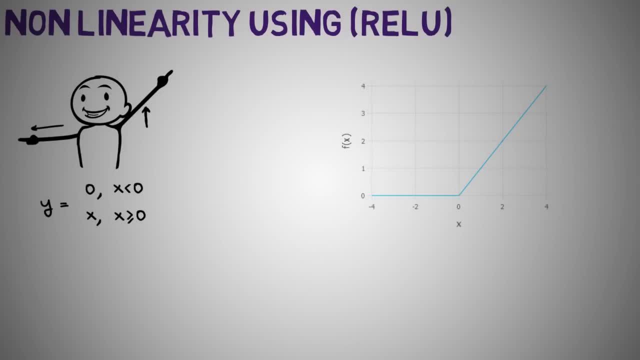 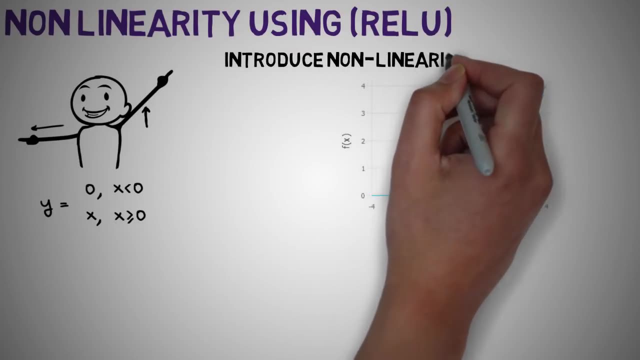 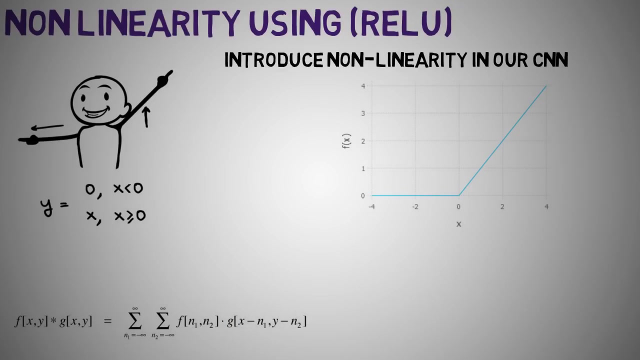 It applies all negative values in the feature map by zero. The purpose of ReLU is to introduce non-linearity in our CNN, Since most of the real-world data we want our CNN to learn would be non-linear. remember that convolution is a linear operation, or rather an element-wise matrix of multiplication. 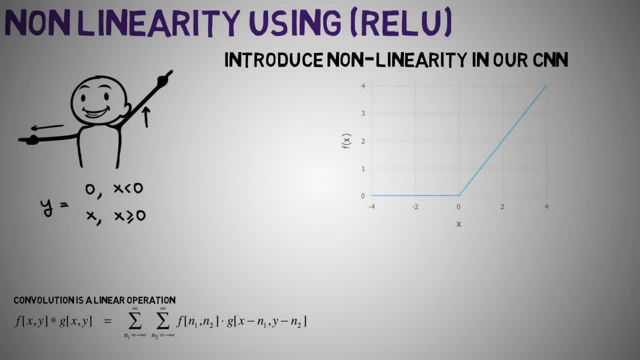 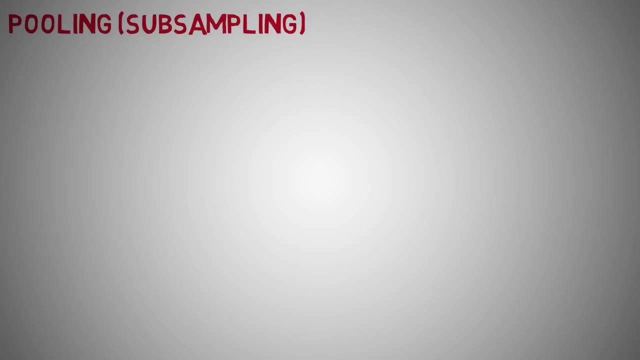 and addition. So we account for non-linearity by introducing a non-linear function like ReLU. Other non-linear functions are the following: ReLU has been found to perform much better in most situations The pooling step. spatial pooling, also known as sub-sampling or down-sampling, reduces the 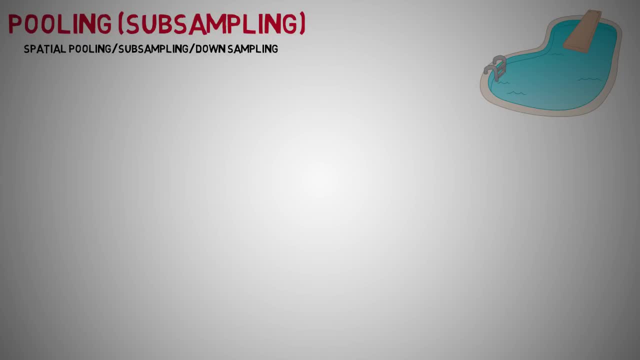 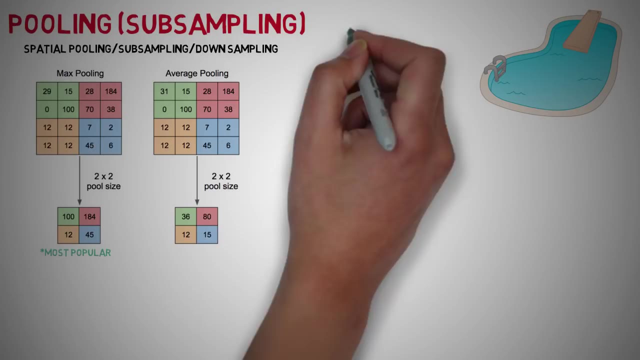 dimensionality of the feature map, but also retains the most significant information. There are various types of pooling, such as max pooling, average pooling, sum pooling, amongst many others. In practice, max pooling has been shown to work better. So what is max pooling? 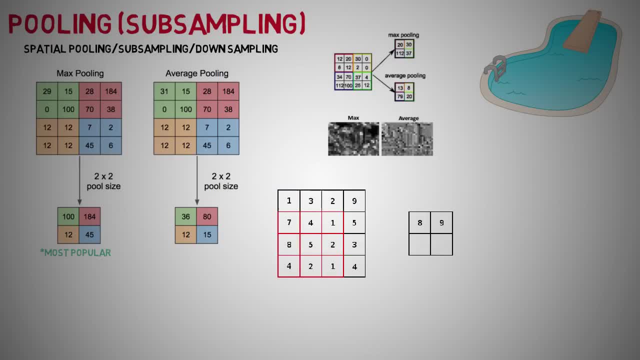 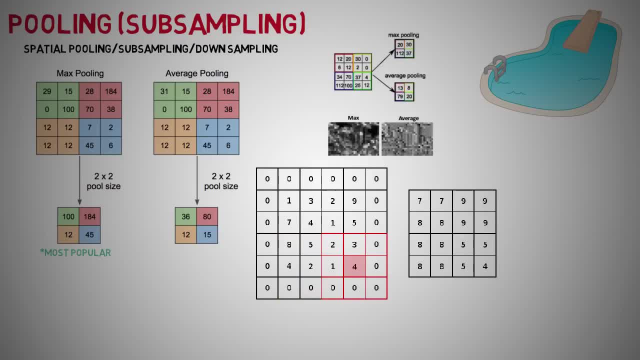 Well, max pooling is when we define a spatial network. So what is max pooling? Well, max pooling is when we define a spatial network. A spatial network has to be labeled, for example, a 2x2 window, and take the maximum element. 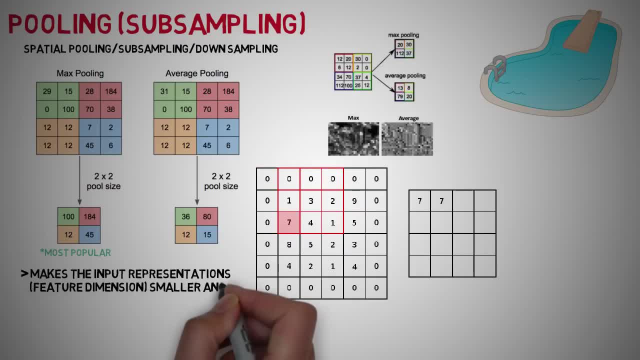 from the rectified feature map within that window. This reduces the dimensionality of our feature map. Some benefits of pooling are that it makes the input representation or feature dimension smaller and more manageable. It also reduces the number of parameters and computations in the network before controlling. 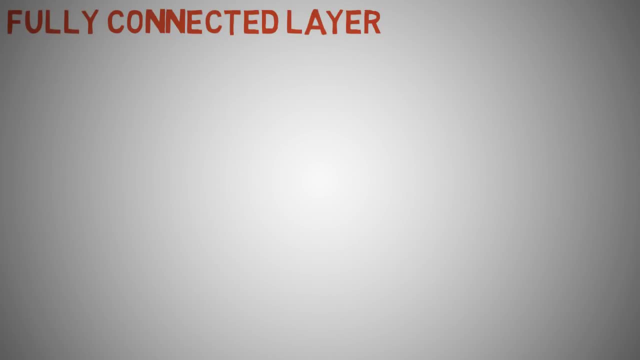 over fitting Fully connected layer. The fully connected layer is a traditional multi-layer perceptron, like we discussed in our ANN lecture, ANN lecture- but that also uses the softmax activation function in the output layer. The term fully connected implies that every neuron in the previous layer is connected. 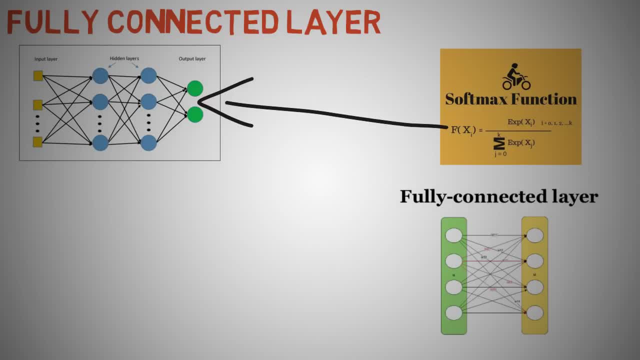 to every neuron in the next layer. The output from the convolutional and pooling layers represent high-level features of the input image. The purpose of the fully connected layer is to use these features for classifying the input image into various classes based on the training dataset. 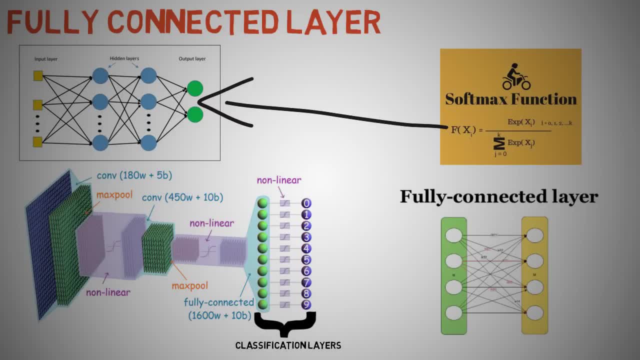 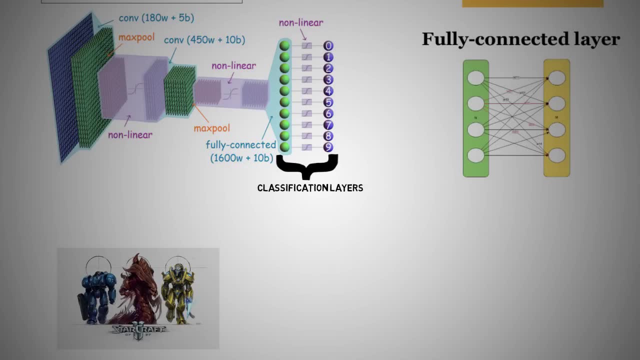 For example, the image classification task we set out to perform has three outputs. So if we look at the game StarCraft, we have the Protoss Zerg and Terrans. Apart from classification, adding a fully connected layer is also a usually cheaper 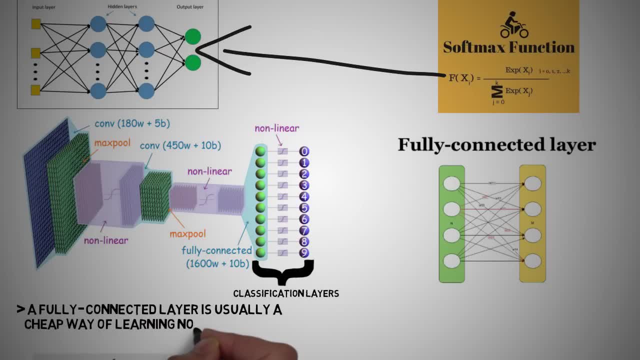 way of learning non-linear combinations of these features. Probabilities that we obtain from the fully connected layer sum to one because of the softmax function. This helps us to distinguish a bit more easily the output of the CNN. So if the output is 60%, dog. 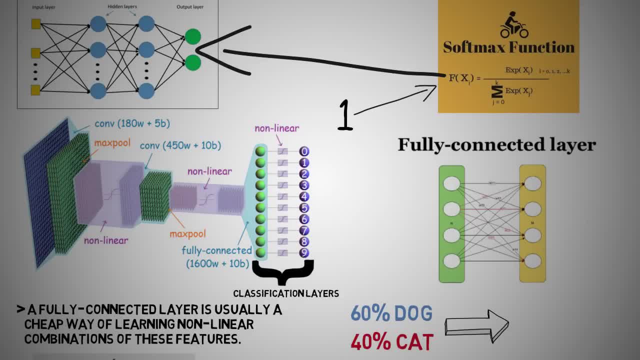 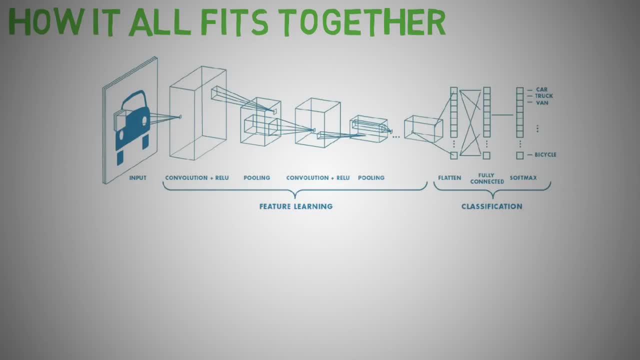 Or 40% cat. By a majority vote, we determine that the output is possibly a dog. How it all fits together? As discussed earlier, the convolution and pooling layers act as feature extractors from the input image, while the fully connected layer acts as a classifier. 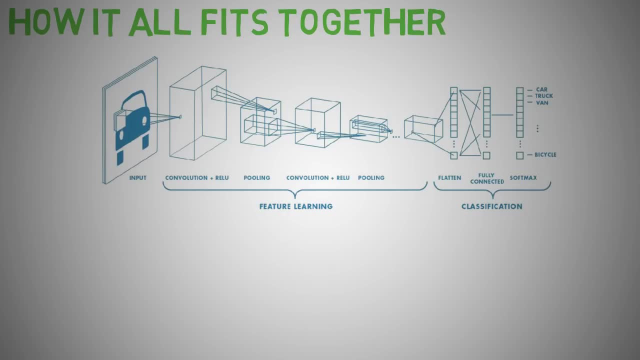 From this image you can see how it all fits together. We have multiple convolution, ReLU and pooling layers to extract the best features. There can be numerous of these layers in which we feed them into a fully connected network Where we get the output of our dog. 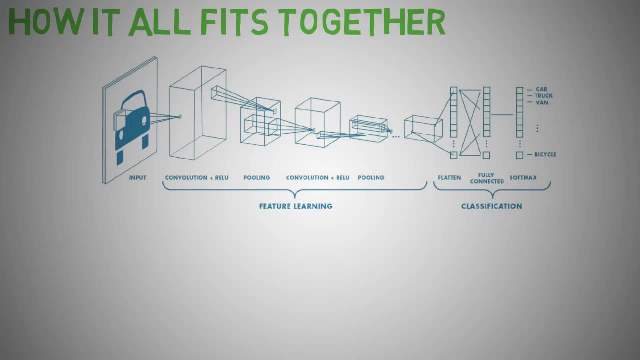 Where we get the output of our CNN, Which is a set of probabilities of what our objects are in our region of interest. So we set our input image and our target vector predicts that we have a marine in our target vector. Training a convnet deserves a video on its own, but let's briefly discuss the process. 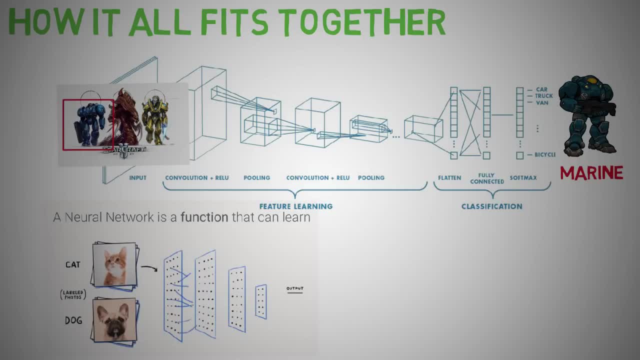 So convnet training essentially means that all weights and parameters of the convnet are now optimized to correctly classify images from the training set. We can use backpropagation for this. When a new, unseen image is input into the convnet, the network could go through the. 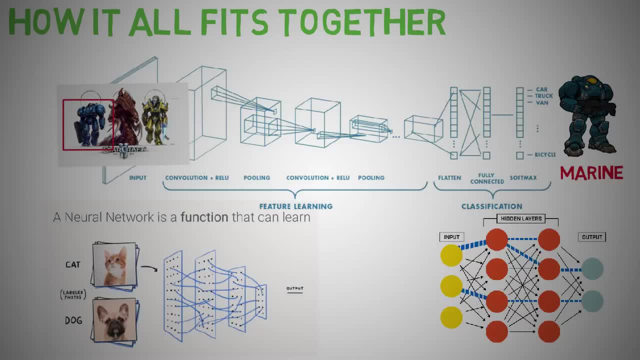 forward propagation step and output the probabilities for each class For a new image. the output probabilities are calculated using weights which have been optimized to correctly classify all the previous training examples. If our training set is large enough, the network will hopefully generalize well to new images. 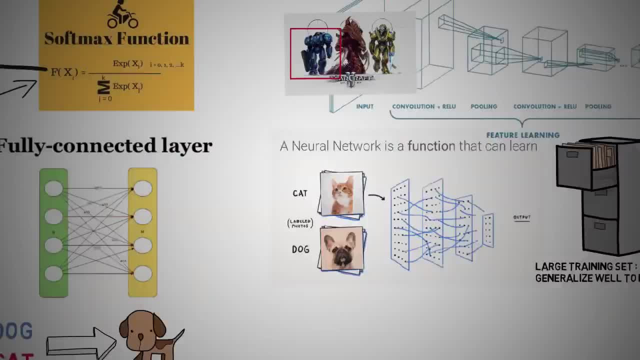 and classify them into correct categories. Convolutional neural networks have been around since the early 1990s. We discussed the LeNet earlier in this video. Convolutional neural networks have been around since the early 1990s. Convolutional neural networks have been around since the early 1990s. 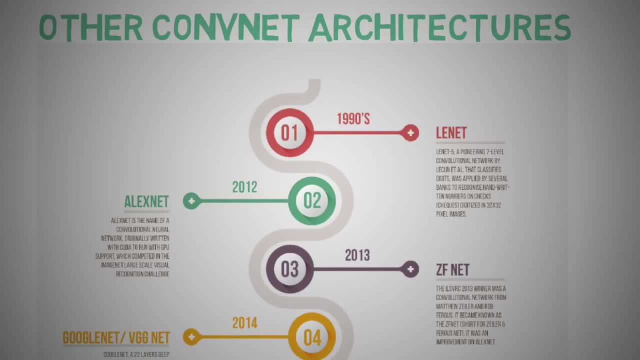 We discussed the LeNet earlier in this video. Convolutional neural networks have been around since the early 1990s. We discussed the LeNet earlier in this video. We discussed the LeNet earlier in this video. We discussed the LeNet earlier in this video. 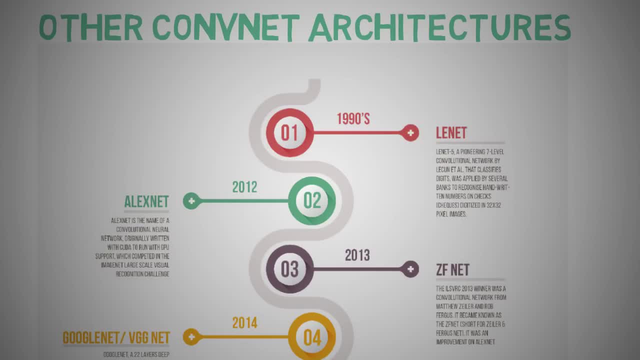 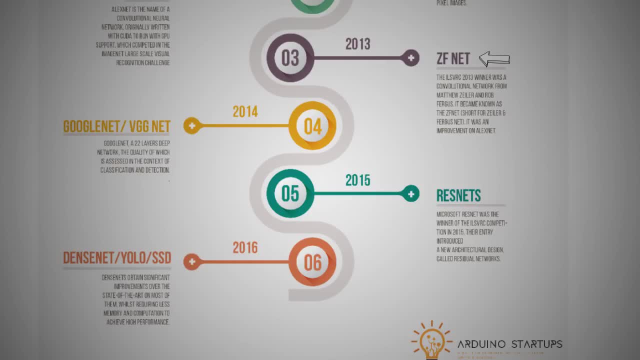 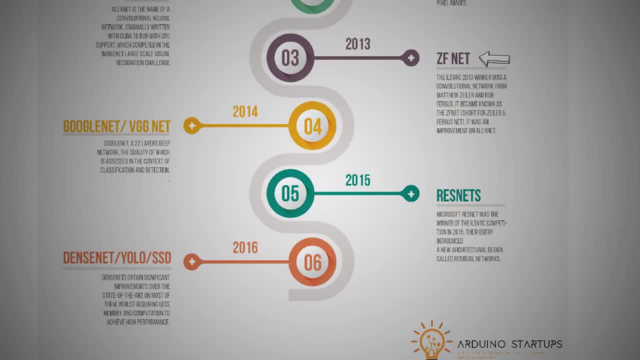 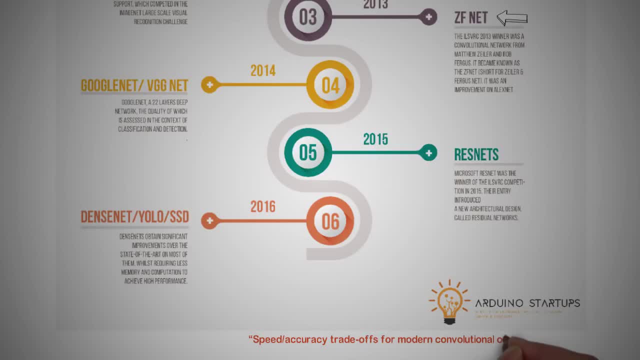 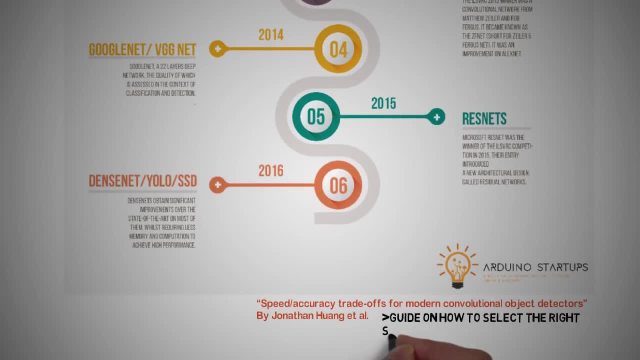 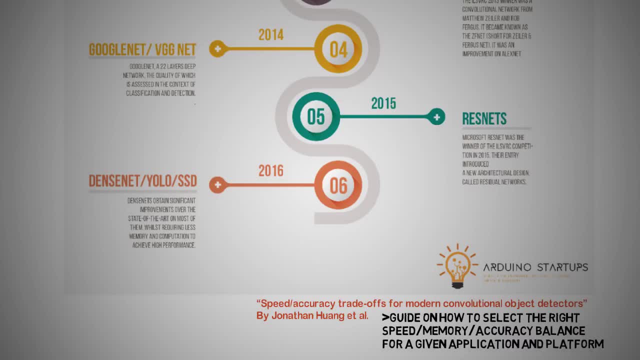